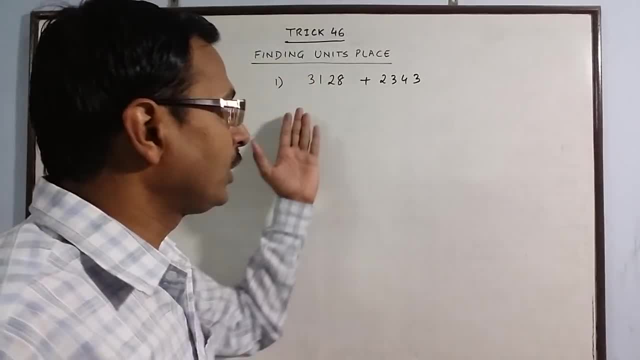 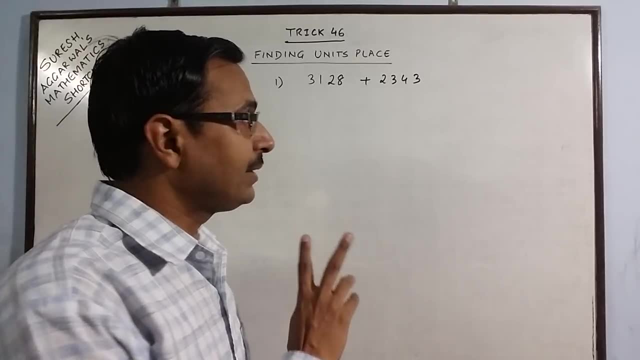 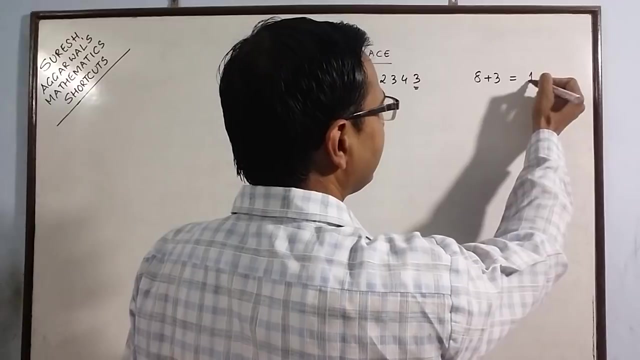 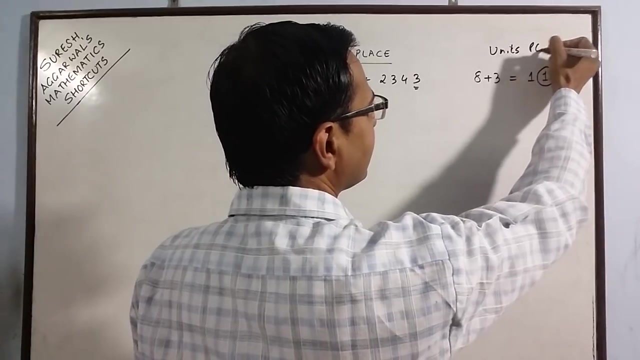 this is very, very simple, because there is no need to add the entire number for finding the unit's place. You just need to add the unit's place of the two numbers. 8 plus 3 is 11, and the unit's place of this sum will give you the unit's place of the entire. 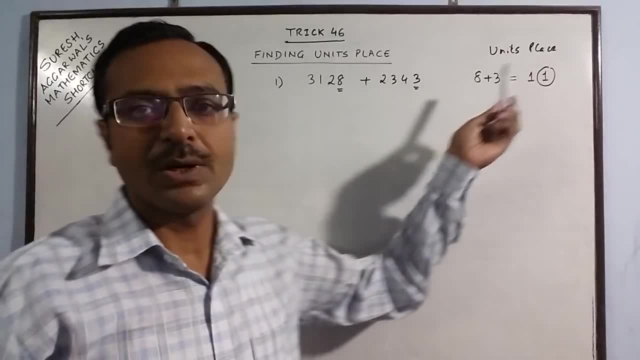 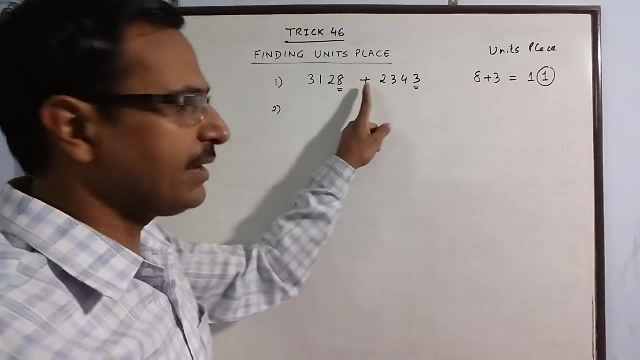 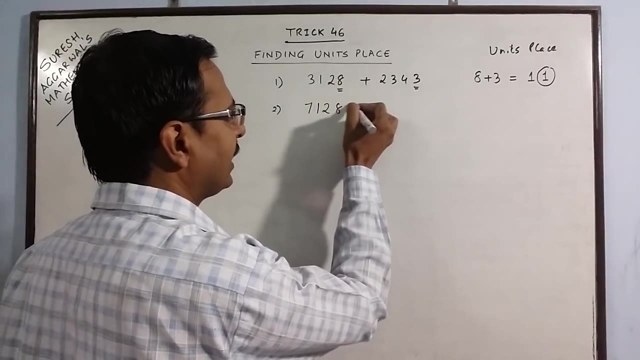 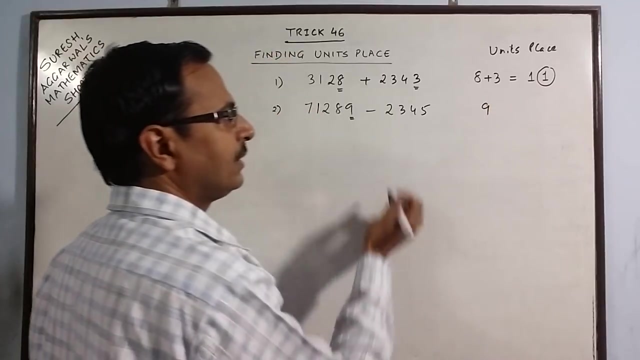 problem. So the unit's place of this sum is 1.. Now, similarly, when the question is based on difference, then you have two different problems here. Suppose we have the question 71289 minus 2345.. Now this unit's place is 9 and this unit's place is 5.. So the difference here is 4. 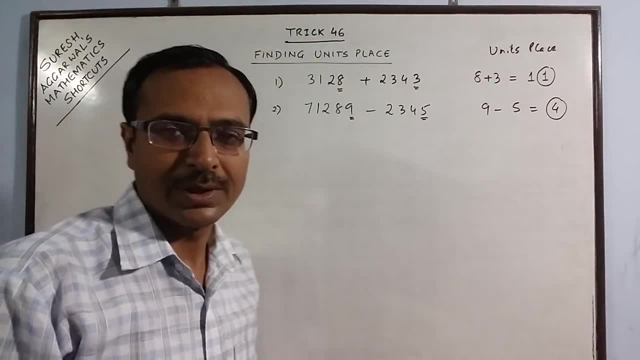 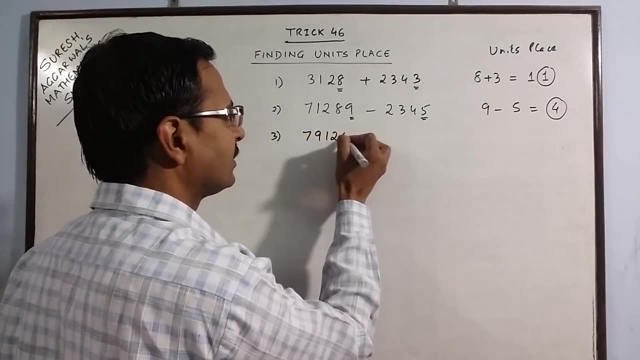 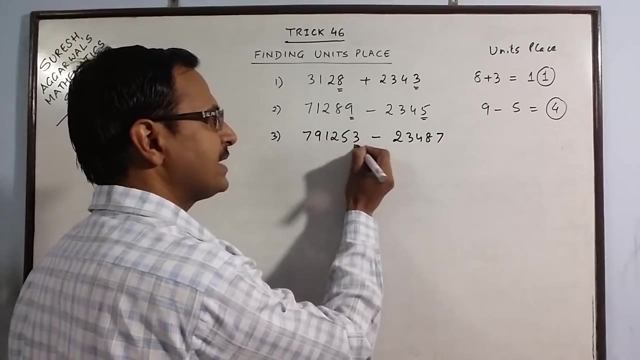 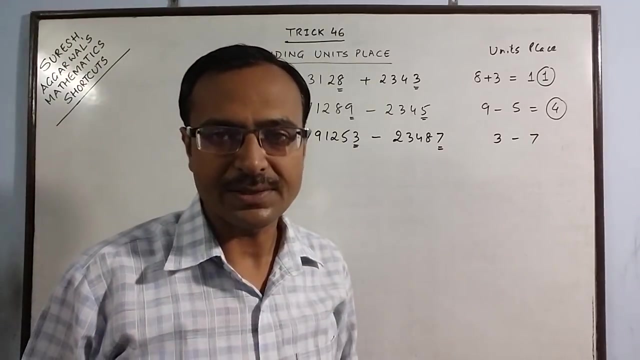 which is the required solution. But when this unit place- suppose you have the problem as this: minus 23487.. Now this unit's place is 3 and this is 7. So the difference of these two will give you a negative number, which cannot be the answer. So what you do is you just put 1 before. 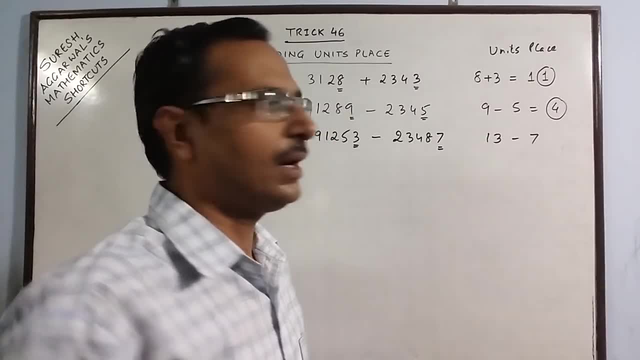 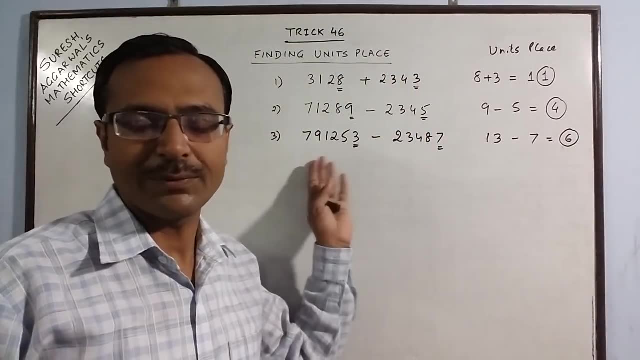 this number 3.. So that it becomes 13. and now the difference of 13 and 7 is 6, which will give you the unit's place of the difference of these two numbers. So the difference of these two numbers will give you the unit's place of these two large numbers. So you see, there is no need to add the. 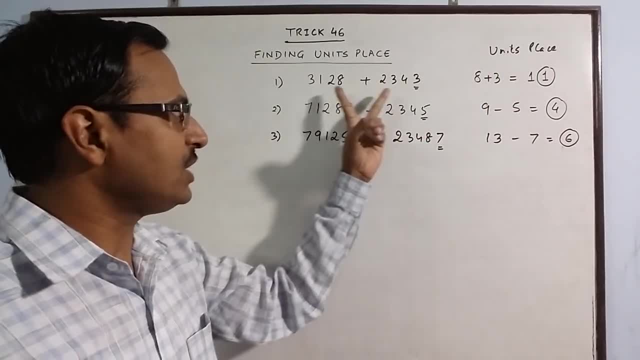 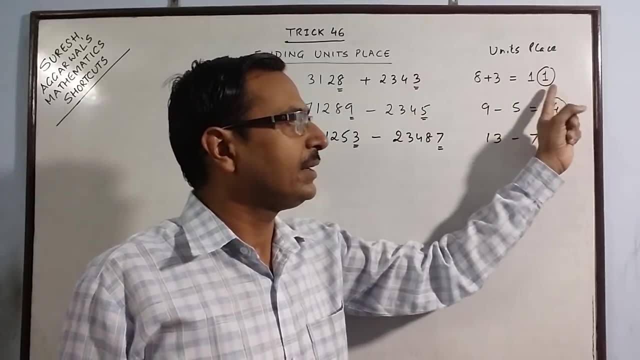 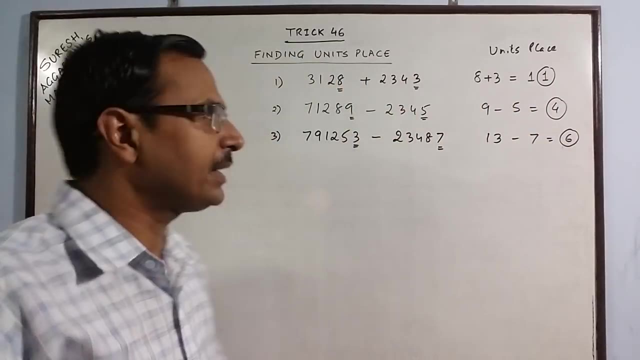 entire numbers to find the unit's place. In addition, there is no problem even if this unit place is smaller than this one. you can add the two and if you get a two digit number, then the unit's place of this sum will give you the unit's place of the problem. But in case of difference, 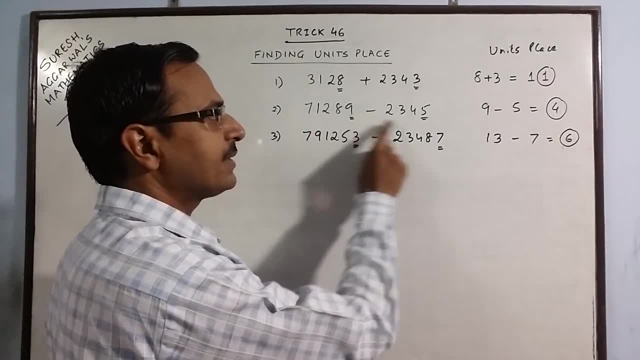 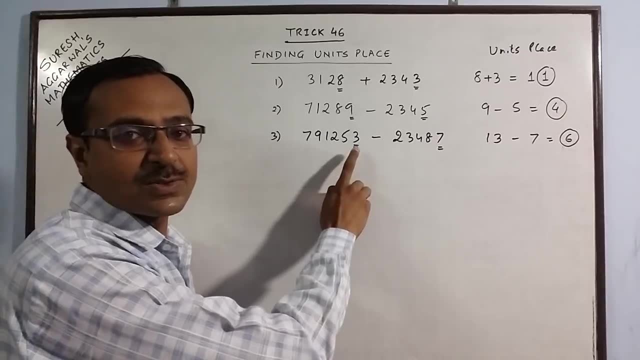 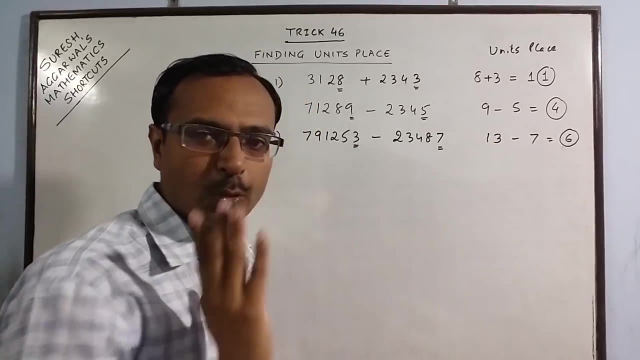 you need to see. if this is greater than this, then the solution is very simple: just subtract and get the unit's place. But if this is smaller than this one, then you have to convert this 3 into 13.. So you have to put 1 prefix 1 before this unit's place and then subtract. 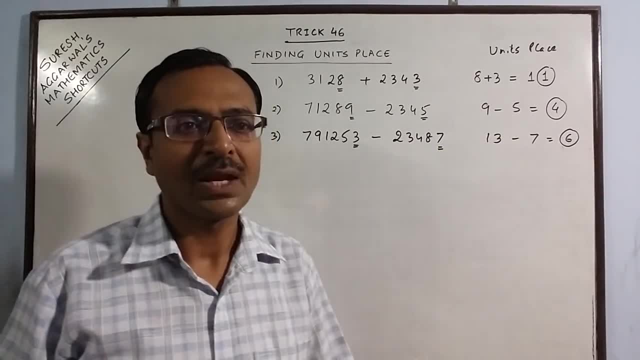 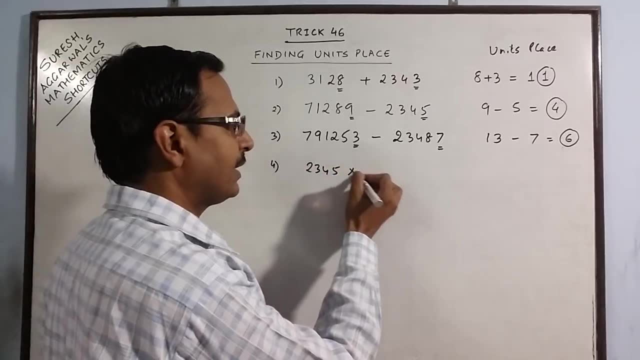 7 to get the unit's place of this difference. Now, coming to product, suppose you have 2, 3, 4, 5 multiplied by 7, 2, 5, 1 multiplied by 3, 4,, 8,, 9.. 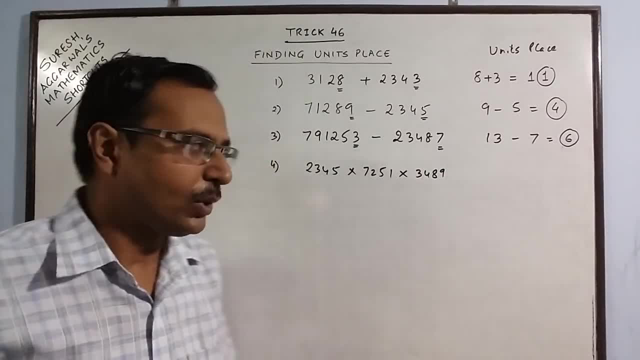 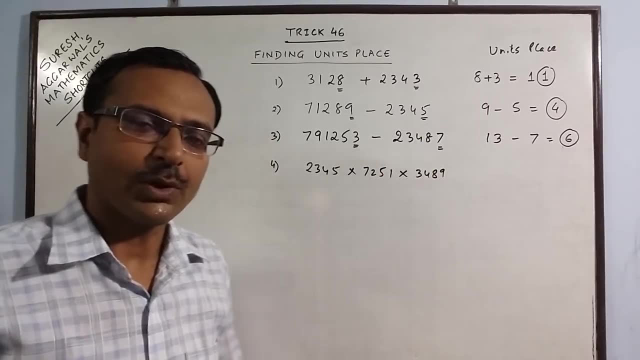 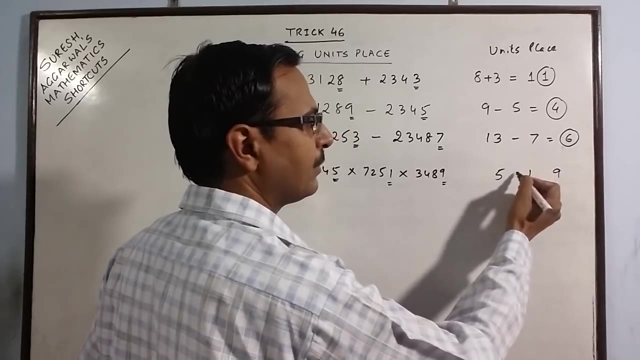 Now, this is a very large product and if you are asked to find the unit's place of this, then obviously you cannot multiply these numbers and arrive at the unit's place. So what you do is just take the unit's place of the 3 numbers- 5, 1 and 9- and multiply these 3,. 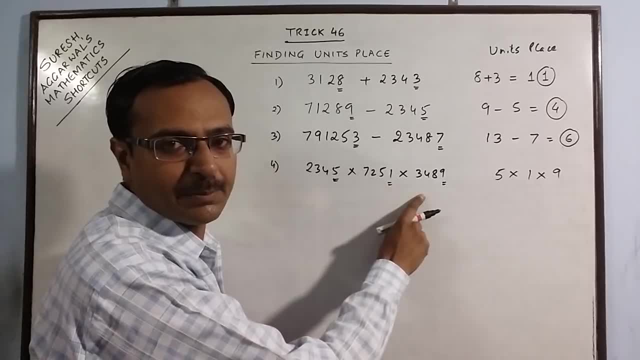 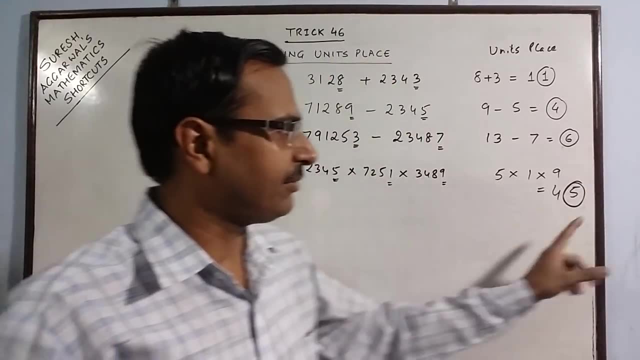 because there is a multiplication operation in between these 3 numbers. So multiply these 3, you get 45, and take the unit's place. So answer is 5.. Now if you want to find the unit's place of this, then you have to find the unit's place of this. 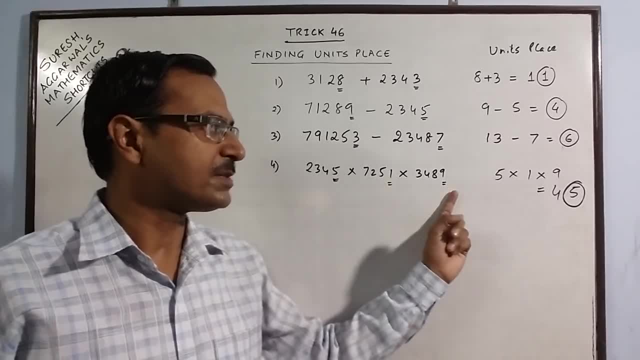 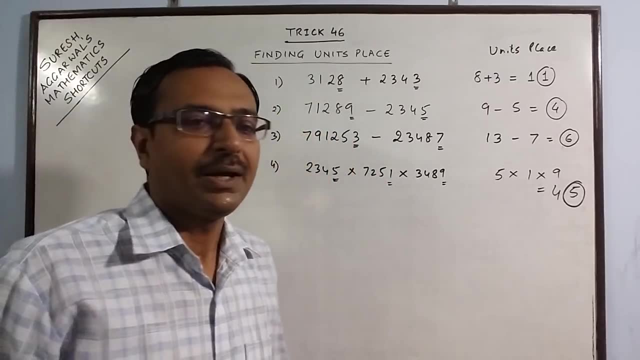 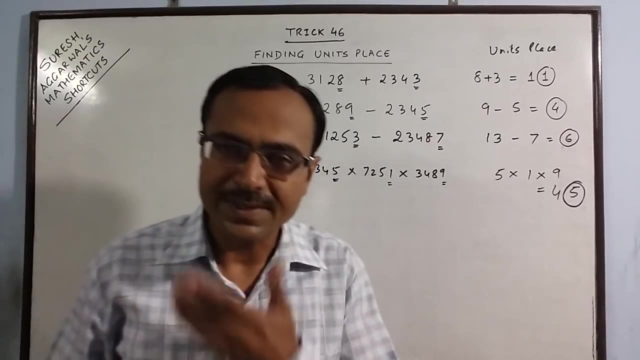 product. So in case of product also, you just need to multiply the unit's places of the numbers to get the unit's place of the product. So sum difference and product. Now come to the most important part, which is asked in most of the competitive exams. 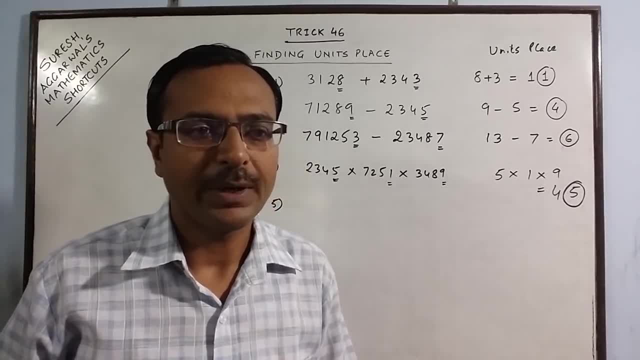 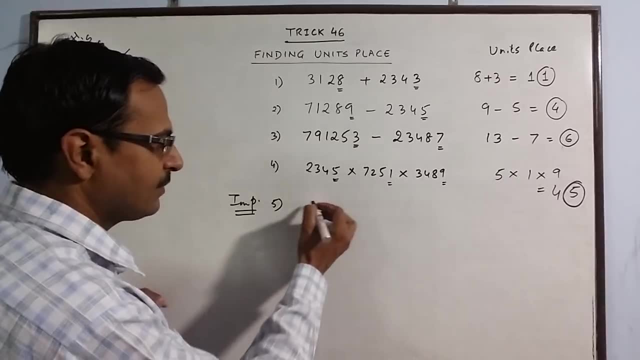 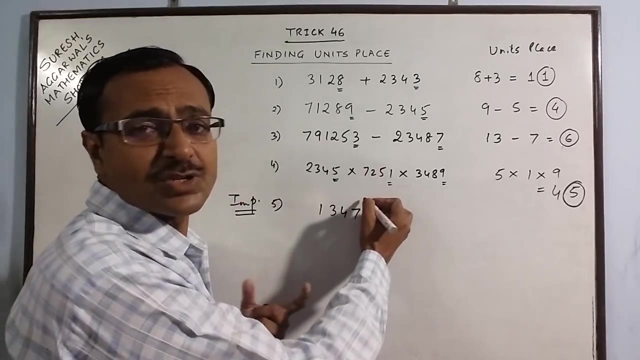 that is, in either in NTSC or railway recruitment or any SSC exams, you will find these type of questions. to find the unit place of: say we have 1347 raise to power. say we have a large power now so that you cannot expand this power. 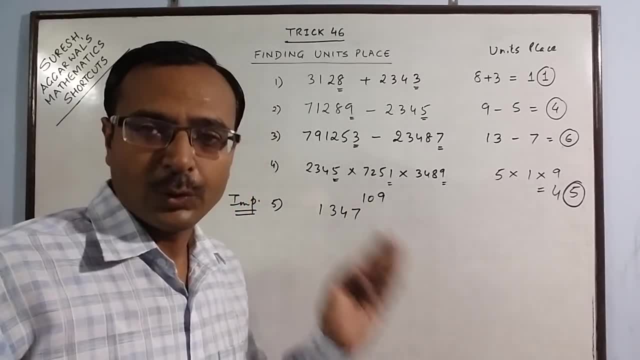 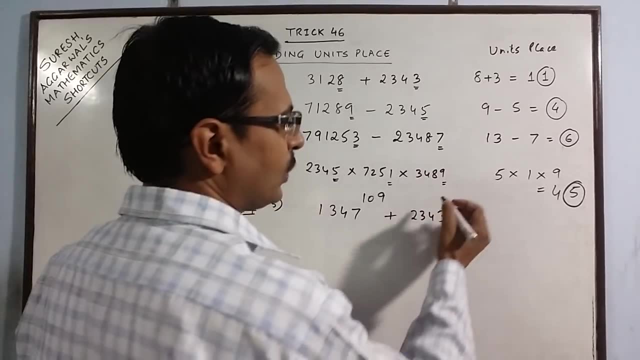 Now obviously there has to be a shortcut to find this unit place now. And we have another number, 2343, and now another power, say we have 27.. Now 1347 raise to power 109 plus 2343, power 27,. 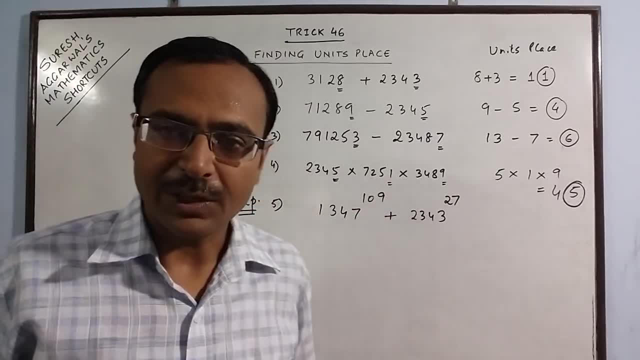 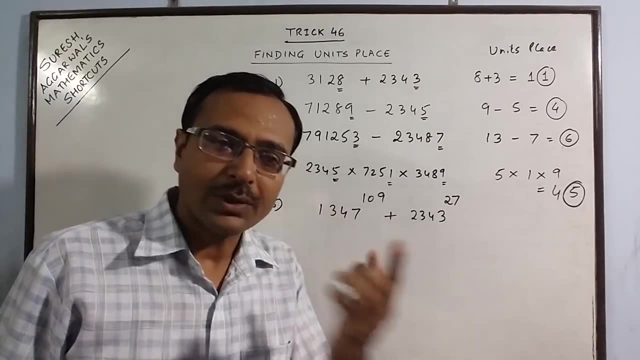 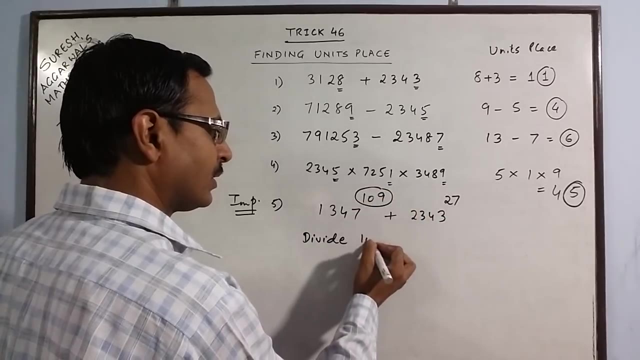 no one can calculate, obviously, this. it is a very, very large calculation. So now I am going to tell you how to find the unit place of this sum. Now, the shortcut for this is what you do is you divide this power by 4,. 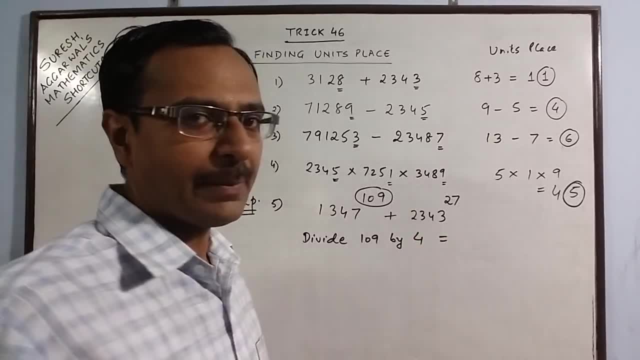 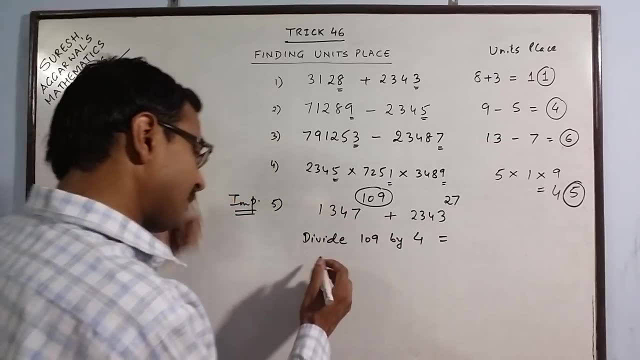 this is the standard number 4.. So you have to remember that whenever you have to find the unit digit in which power is given, then you have to divide the power by 4.. Okay, Then similarly divide the other power, 27,. 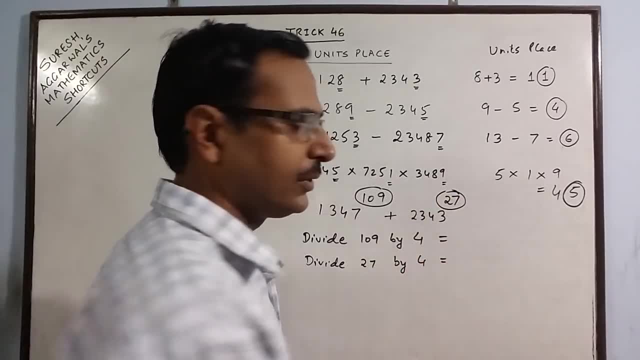 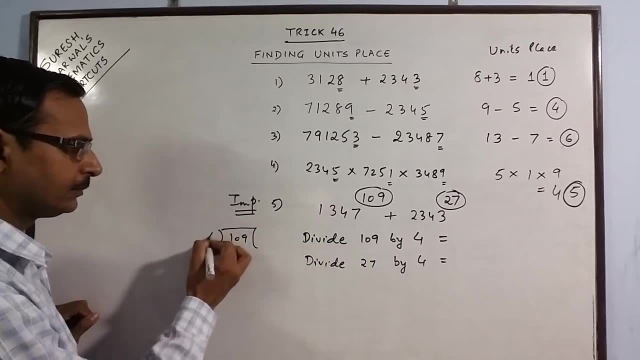 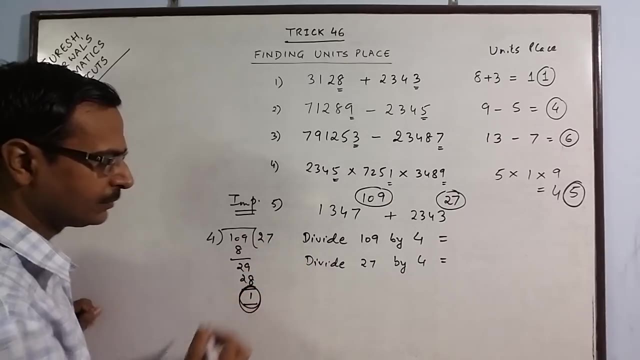 27 by 4.. 4 is standard. You have to always divide by 4 only. Now what happens is, when you divide 109 by 4, you get 1 as the remainder. Now remainder is 1.. Similarly, when you divide, 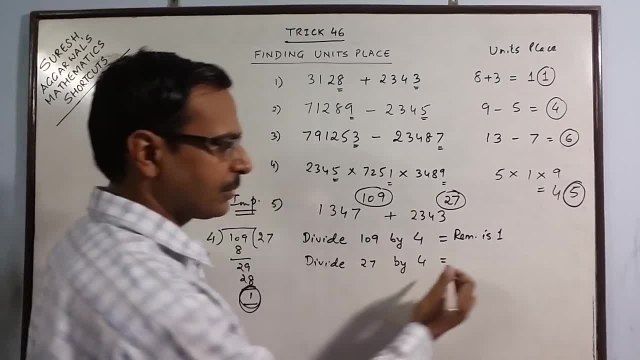 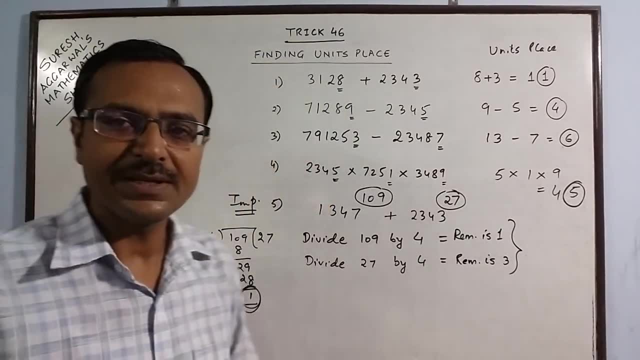 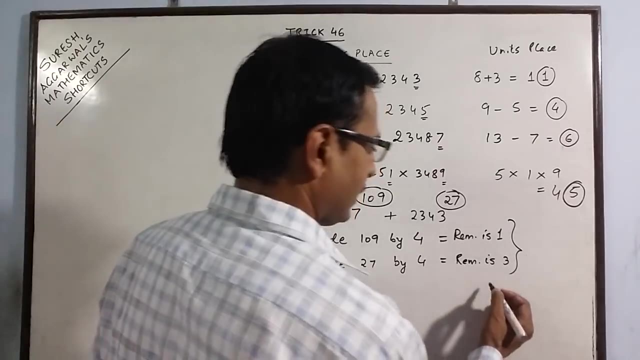 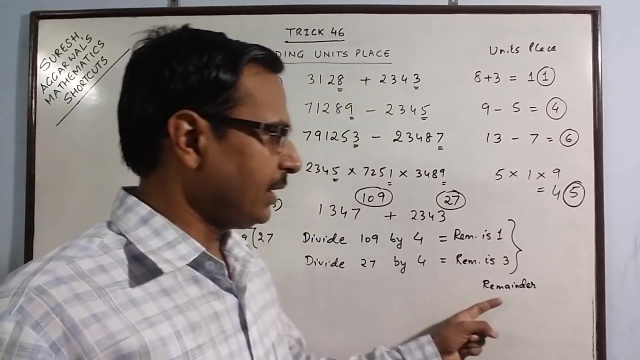 27 by 4.. So 4 is 24.. So remainder is 3.. Now you have to remember these remainders. On the basis of these remainders only you will get your solutions. So now there is a small table which you have to remain in your mind: Remainder and the power If the remainder. 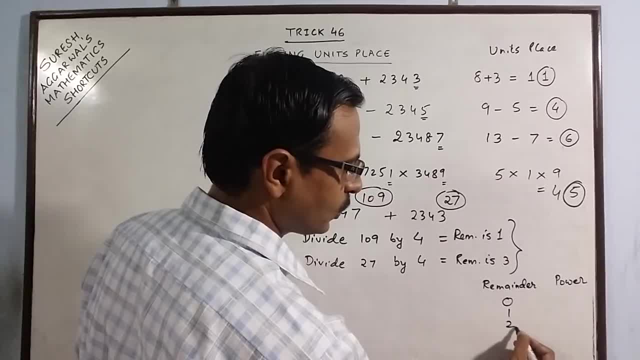 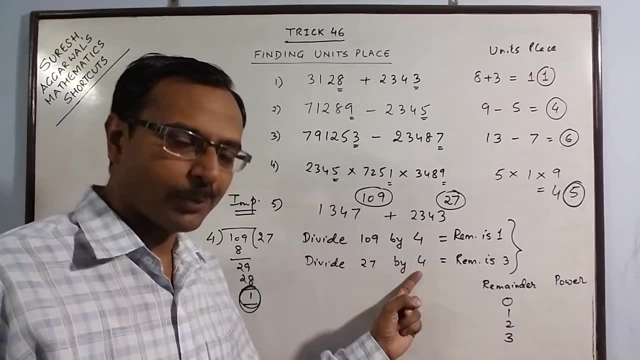 is 0. If the remainder is 1, remainder 2, remainder 3.. Because obviously remainder cannot be 4 or greater, because we are dividing by 4. So it cannot be 4 or more than 4. So we are taking. 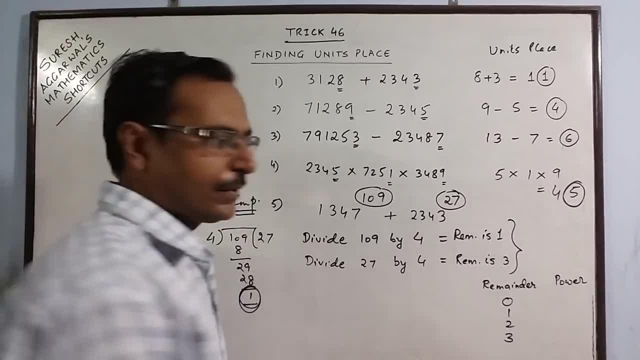 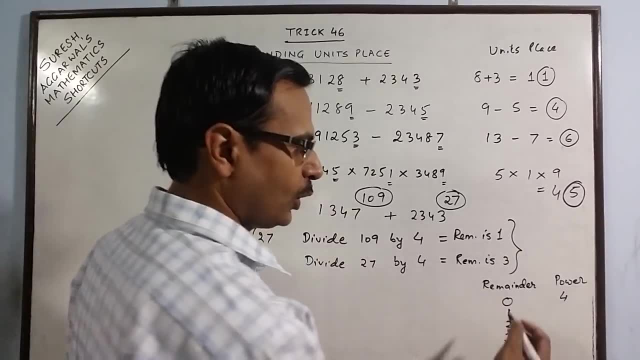 remainder: 0,, 1,, 2,, 3.. So if the remainder is 0, then you take power as 4.. And in all other cases the remainder and power remains same. So remainder is 1, power is 1, remainder. 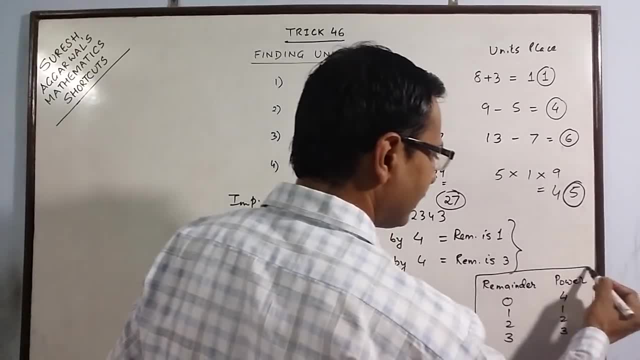 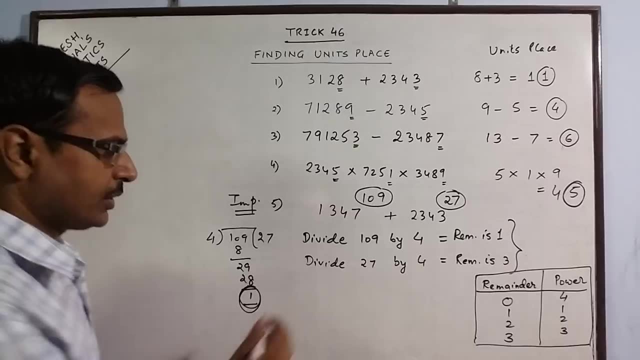 is 2, power is 2,. remainder is 3, power is 3.. Now, this is a small table which you have to remember for finding the remainder. So let us take the units place of this question. Now the required solution- units place- is given. 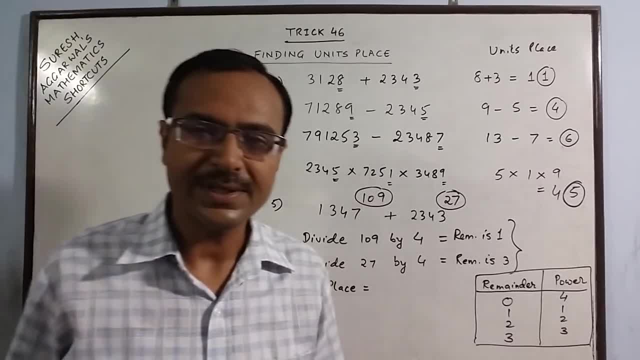 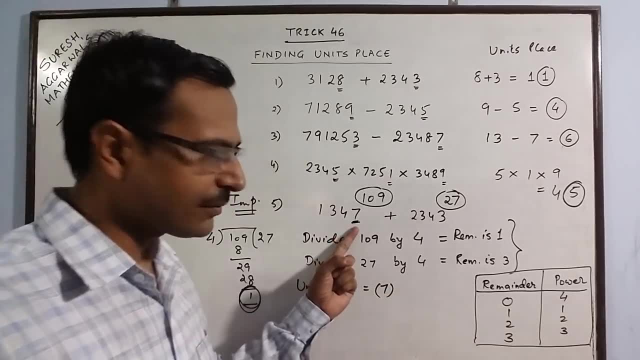 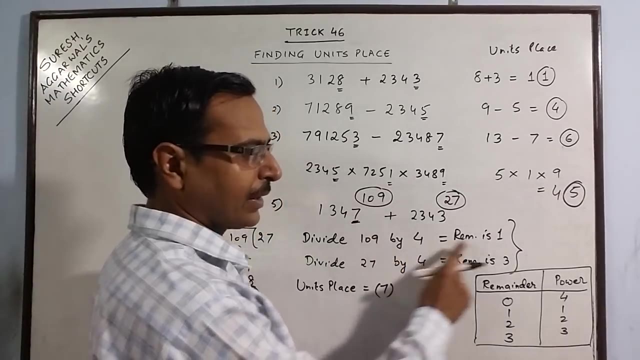 by Now. there is a direct formula for this. What you do is you take the unit place of the first number, 7. Unit place of the first number, and you see the remainder when it is divided by 4.. The power is divided by 4. The remainder is 1.. So when the remainder is 1, 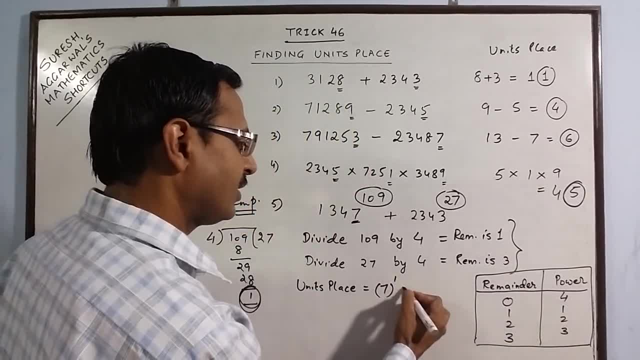 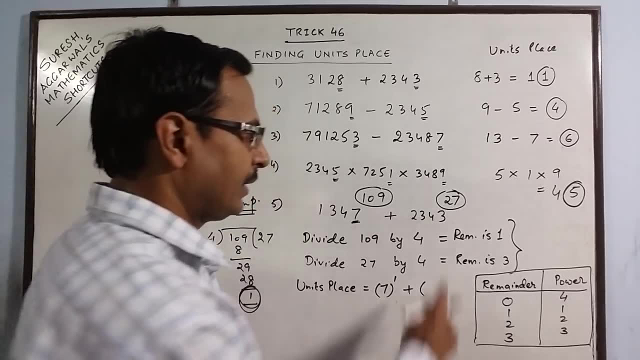 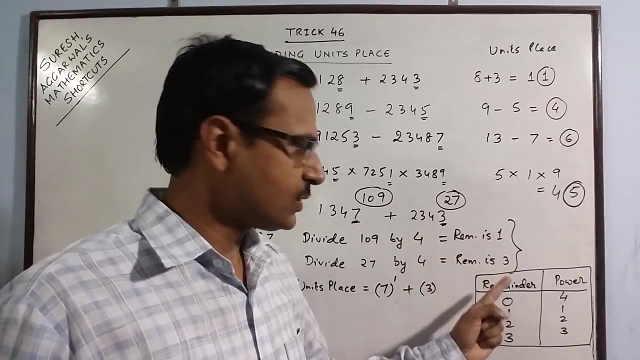 the power is also 1.. I raised 7 to the power of 1. And now there is a plus sign in between. The unit place of this number is 3. And when I divided 27 by 4, I got the remainder as 3.. So when remainder?